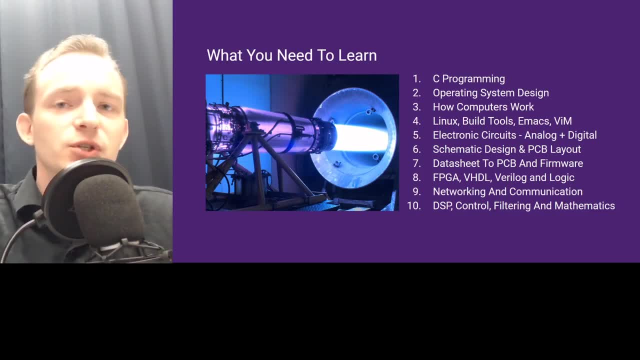 And embedded systems. it can be very confusing when you first get started. You just sort of you get lost in questions like: do I need to learn Arduino, Do I need to learn STM32? Or do I need to learn C, Or do I need to learn some other language? 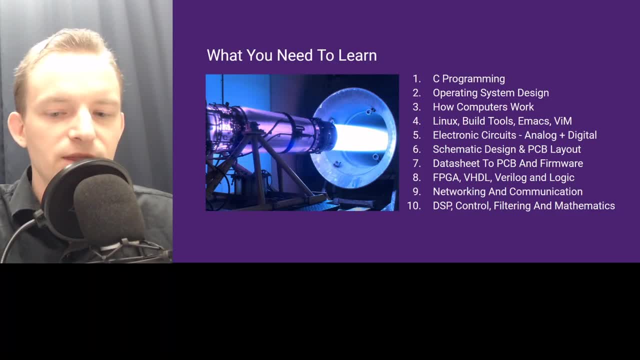 And people get confused, And I think that the main thing for you to do is kind of you're getting started, like if you ask a question, do I need to learn Arduino? You're really kind of starting at the wrong end of things. 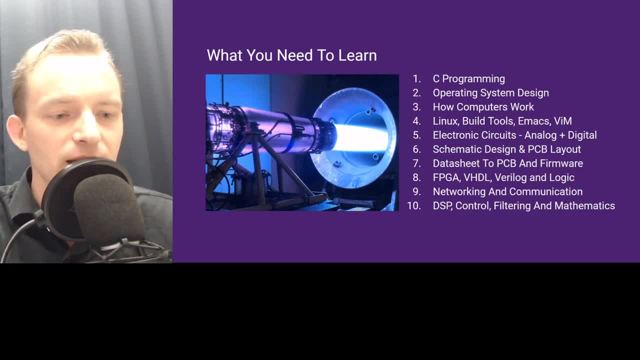 Because you need to start from the beginning and ask yourself: what is it that you need to, what is it that you want to create? And even farther towards the beginning, you need to ask yourself: like who do you want to create it for? 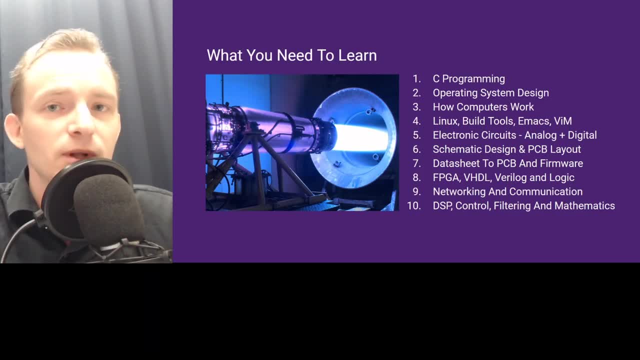 And you achieve that by kind of by getting in communication with people and figuring out what it is that you want to create, And then from there you start learning. But I've broken down embedded systems into 10 areas that you need to learn. 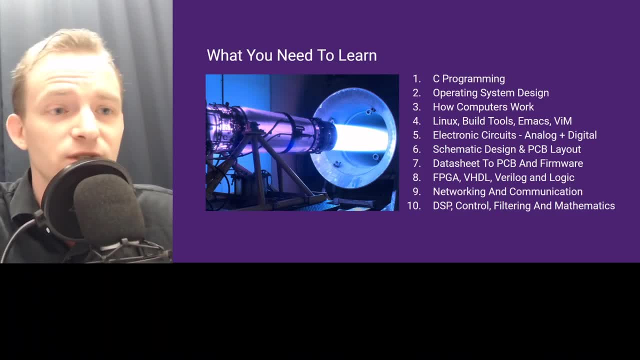 And I'll explain to you why you need to learn, And hopefully you get some tips during this live stream. And let's just get started. So one of the the number one step when it comes to embedded systems is really getting comfortable programming the C programming language. 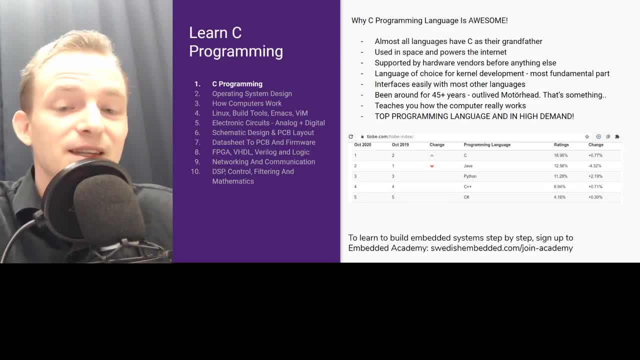 And the C programming language is once again number one in terms of the languages that are most popular for programming embedded systems. It is getting more and more popular because it's used in things like flight control. It's basically any, any kind of little device that doesn't run any operating system, that just uses a microcontroller where you program, put the program directly on the chip and it runs directly on the chip without any assistance from any operating system. 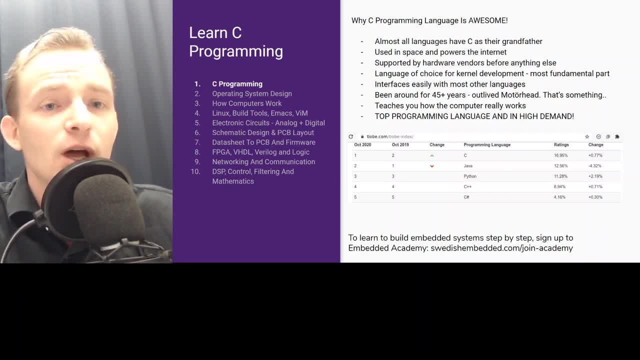 In almost all languages. if you, if you really think about it, if you break it down, almost all languages that we have today they're based on C to some extent. So they are, they're, they're kind of. they are either derived in terms of syntax or they have borrowed. 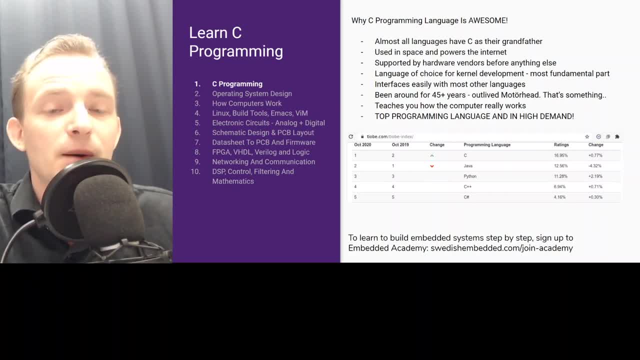 borrowed ideas from C, And C kind of ends up being this: this grandfather language, which which has has created all of this other languages as an ecosystem around it. And C is extremely easy. Like C is the first language that gets supported by a new tool chain, by a new, by a new chip that manufacturer produces. 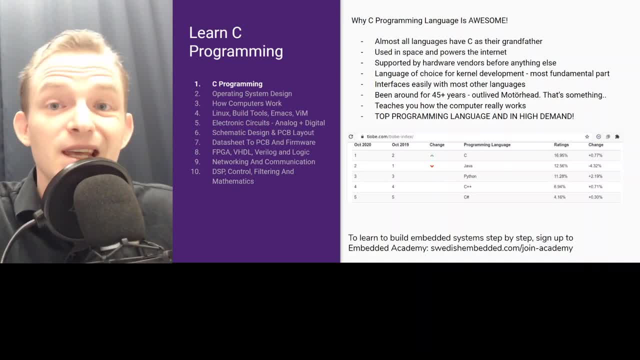 The first thing they do is they make sure that it's possible to program the chip in C, And only only after that do they even focus on C plus plus or or any other language that you can program in. But C is is the ultimate programming language for for small embedded systems. So you really want to get comfortable with with C. It's been around for 45 years. It even outlived Motorhead And that's. that's really cool, because 45 years plus, now it's 48 years since C was created. It was created in 1972, the first version, the first kind of official version, was created in 1972. So it's been around for 45 years. So it's been around for 45 years. So it's been around for 45 years since C was created in 1978. 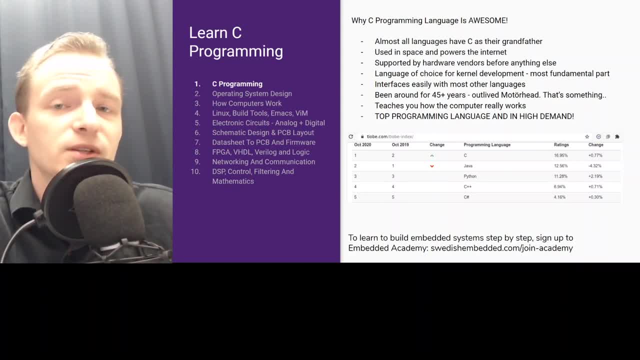 So it's quite a it's quite an old language and it's it's been tested throughout the years and it's still. it's still the most popular language today and used everywhere. So learn C, learn, learn the concepts of C. 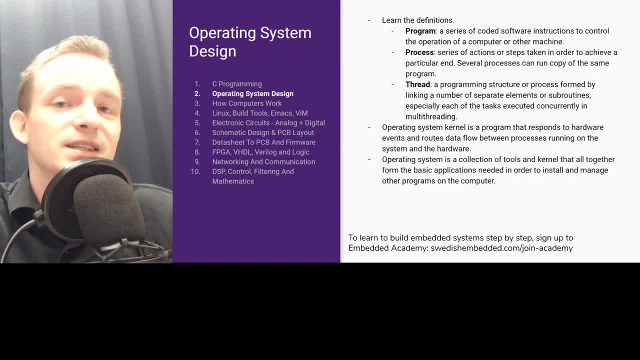 And the next thing you want to learn when it comes to, when it comes to embedded systems, is operating system design. What you will find is that, since you don't have an operating system, you kind of end up implementing certain things in in your 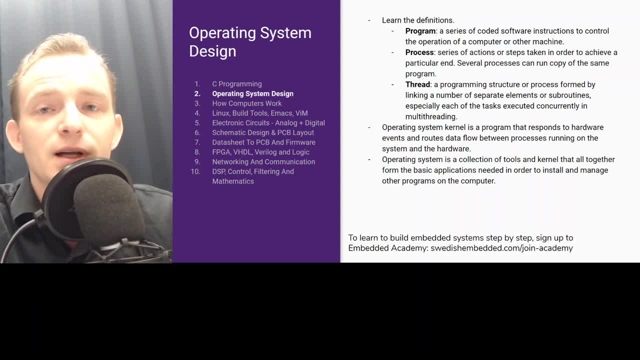 in your software that resemble kind of like the functionality of operating system. So you'll find yourself, for example, writing device drivers. You'll find yourself implementing functionality for reading file systems and all of those things And kind of like. organizing those things together requires you to have an understanding of of operating systems. 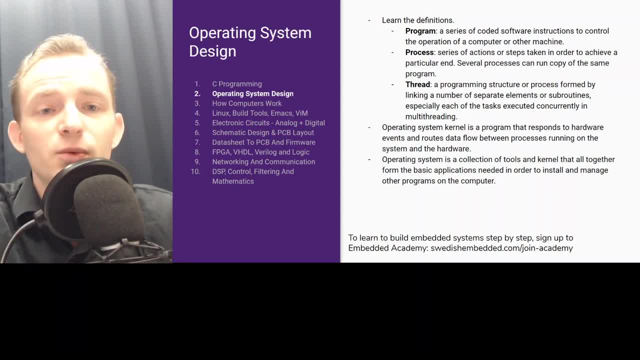 You need to learn the definitions. You need to understand what. what is a program? What is a process? What is a thread? How does the operating system kernel works And what is it how? how does the programs? how do programs communicate with the operating system? 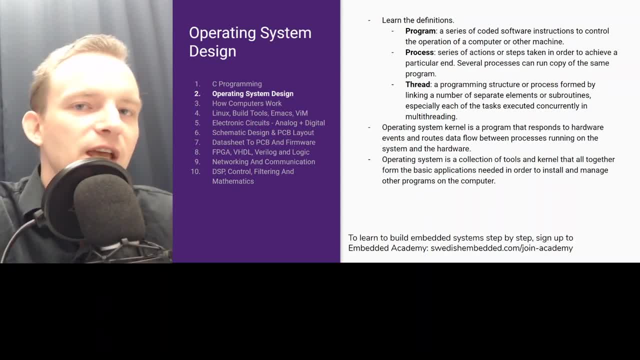 And how does? how does this? how does your code from the application end up in a device driver, Like what are system calls? How? how does the data flow to the, to the actual device? when you write data to a socket, How does it flow to the actual ethernet chip? 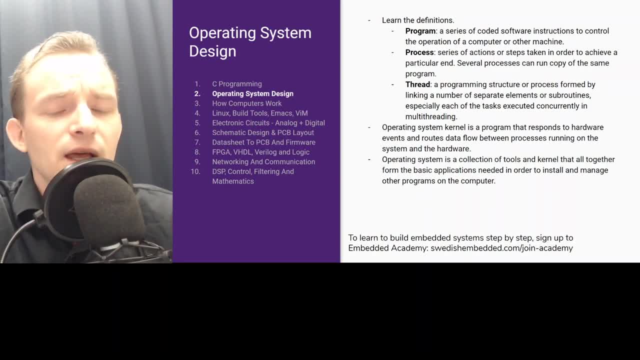 It. it the actual ethernet hardware, and you want to understand this because because when you're working with, with small embedded systems, they're never standard, like like. there's always variations and there's always special cases. Every hardware is created for the particular problem that it's trying to solve. 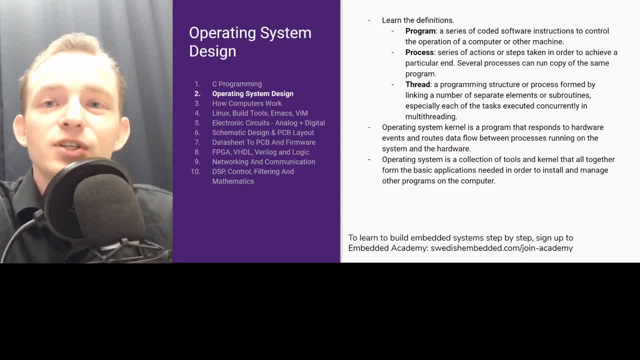 So it's not like buying a laptop. It's more like creating something new and something optimized for solving a particular problem. So you'll find yourself creating a lot of patterns in your code That resemble how operating system works. So it's a very good idea for you to learn operating system design. 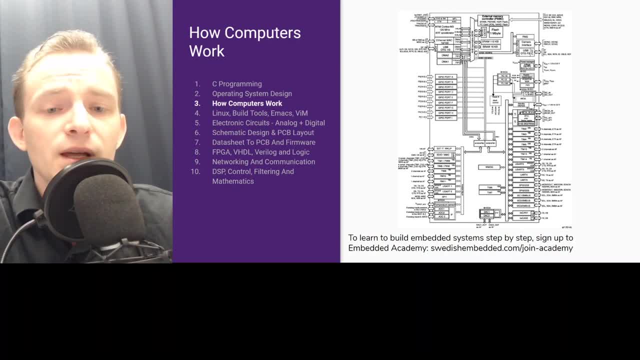 You also need to understand how computers work in general. So if you, if you've started learning, like in the recent years, you're probably most familiar, Like you haven't actually seen the earlier boards that were using external peripherals for almost everything. 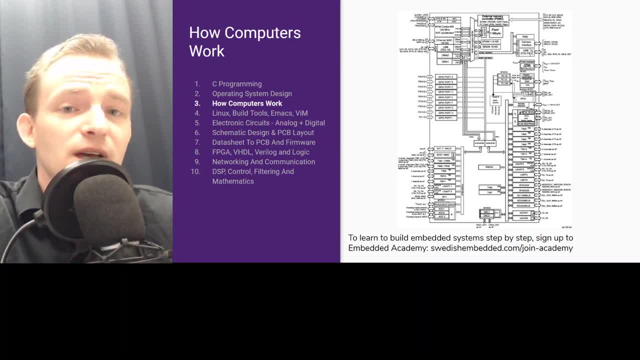 Today we're using microcontrollers. Today we have it a lot easier. today, Everything is put on the same Chip, but the principle of operation is still very much the same as it was 20 years ago or even 30 years ago. It's just that we have evolved the hardware. 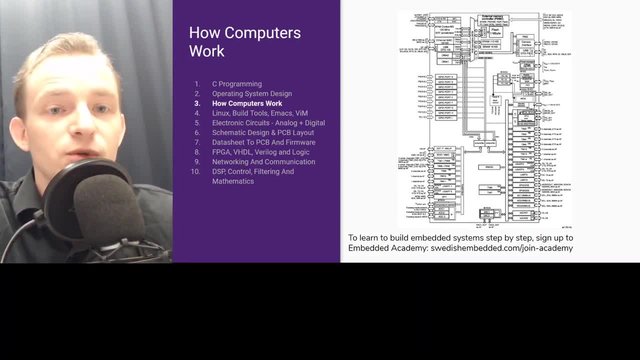 The hardware is a lot more complex today and user user manuals and data sheets can be several thousand pages long. So to kind of find your own way in this huge amount of data about how chips work, it's a good idea to kind of learn. 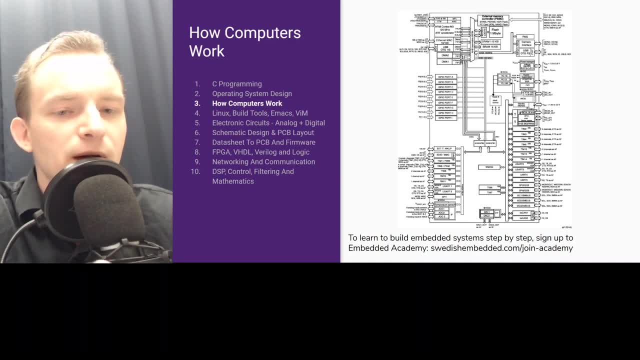 How computers work in general, like how, how does the RAM get addressed and how does the, how does the microprocessor itself like load the code from RAM and actually run the code And how does it communicate with, with the peripherals? So when you understand how computers work, you kind of get a better understanding also of how to structure your code, because when you're writing code and see, very often you're kind of you're kind of mimicking the way that hardware works. 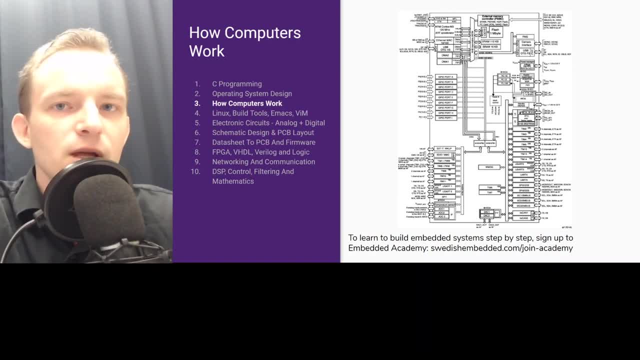 Very much in in C because it's so close to hardware, you don't have abstractions like you would have in C++, you're not hiding so much, so much implementation detail, but instead everything is kind of visible and and because of that you have a very close resemblance between code and how the actual hardware works. and the more you understand hardware, the better you understand how to write code as well. 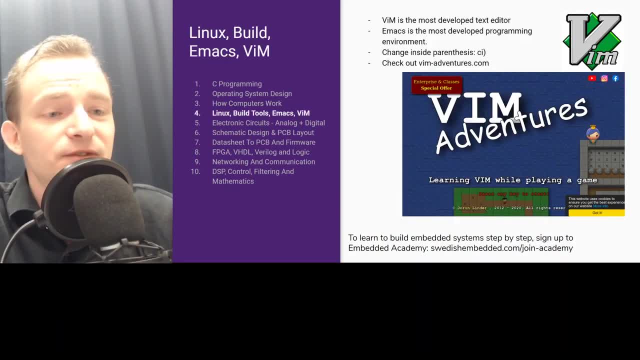 You'll find yourself working a lot in Linux, And The fact is that embedded developers prefer Linux more, and one of the reasons for that is because a lot of embedded systems use Linux when. when it comes to to having an embedded system that actually needs to communicate with the network or has any kind of wireless hardware in it, then you need Linux, because you can reuse a lot of the, a lot of the code that's already available in Linux and you want to get really comfortable with, with the IDE that that is Linux. 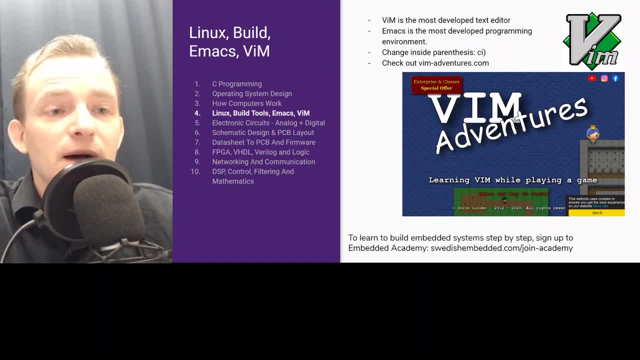 So Linux is like a Linux is like an IDE and it's built out of all these tools that you have available to you. you have text editors, you have compilers, you have command line utilities, you have, you have documentation generation tools. there's so many tools and they all build this, this one integrated development environment, and the cool thing is that you can actually create your own development environment that mimics your way of working, and that's the biggest power of of using Linux. 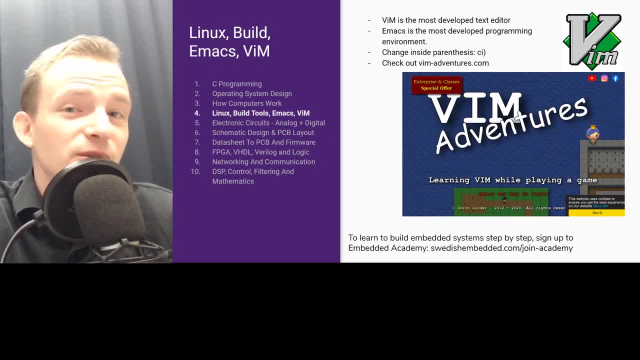 So that's why People People that that program close to hardware. they usually prefer Linux. and it's a good idea for you to learn things like the Vim, the Vim text editor. it's going to be a little bit of a curve, like the first time you start Vim you may be not even going to know how to close it. but as you get a little bit along the learning curve you'll find that you'll be doing things in Vim without even thinking and it's. it's really one of these editors that once you learn it, you don't. it doesn't get in the way, it's just there to to help you. 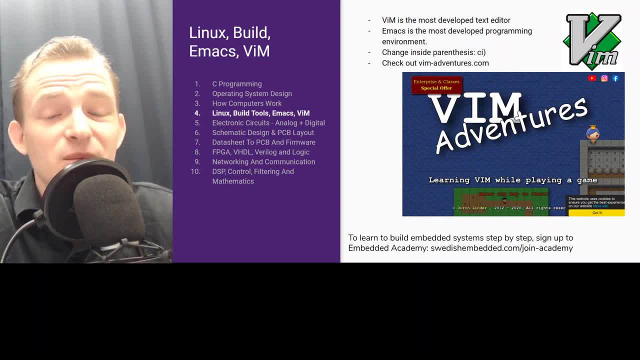 accomplish things. So for example, like simple commands, like CI and then a character, what it means is basically change inside. So C is change, I is inside, and then if you put a parenthesis there, you will just delete. it, will delete anything that is within the parenthesis, and then you can write something else there. 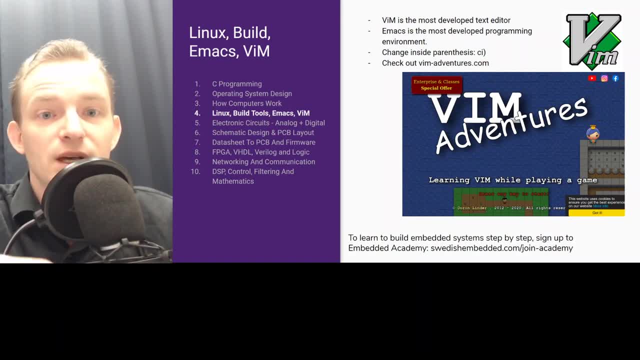 So, for example, if you have function calls, you can use CI parenthesis to just replace all the arguments and it's really quick and Vim has a lot of such commands. One of the best ways to start learning Vim is through a game that is available online. if you go to vim-adventurescom, you can actually play a game and learn Vim as you play the game. 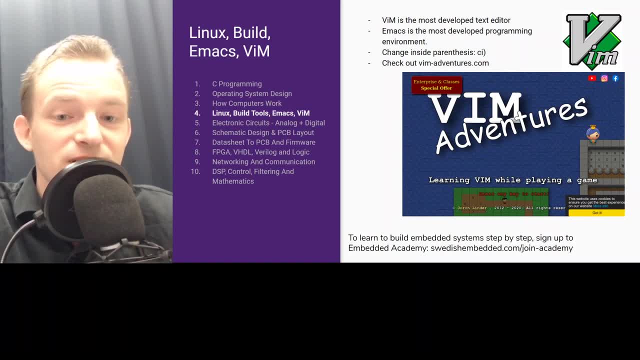 And I've been playing this game when I was learning Vim, when I really wanted to take myself to the next level in using Vim, and I learned so much from this game. It really makes learning Vim a very pleasant experience And actually a lot of fun. 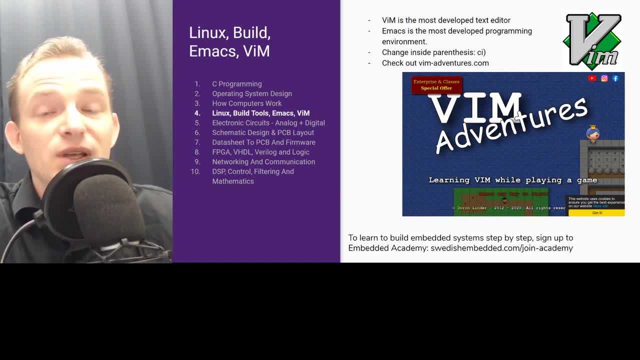 So definitely check it out. When it comes to Emacs, I even converted Emacs to kind of mimic the Vim keybindings because I find that Vim really solved the issue of keybindings. Like, when it comes to keybindings, there's nothing in the world that is better than Vim. 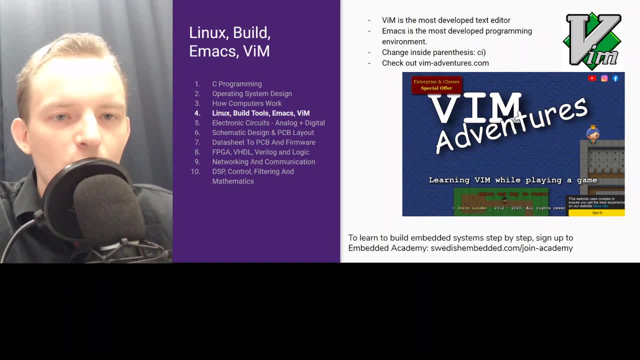 It's really. it's so intuitive and it's so powerful that really like when you start using it, you start to feel like you're actually using it. It's really it's so powerful that really like when you start using it, you start to feel like you're actually using it. 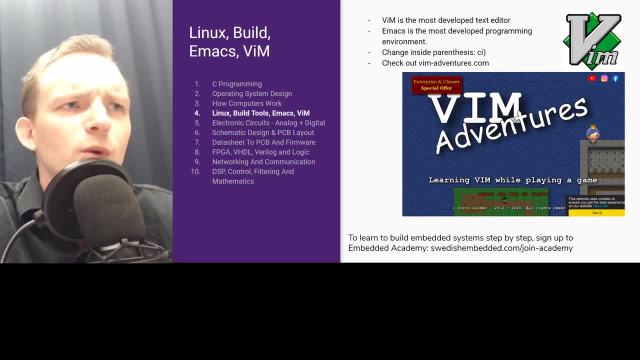 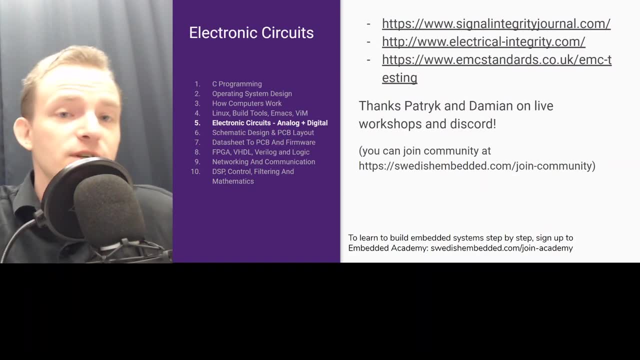 You will never want to go back to any other editor And you'll want to convert every single editor into something that resembles Vim. You also need to learn electronic circuits. There's a lot of good websites, And big thanks to members of our community for sharing these resources. 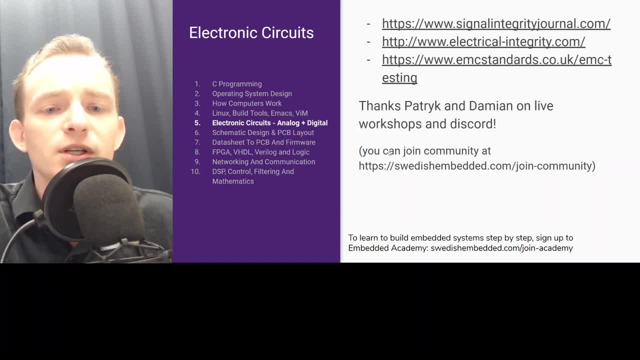 And there's a lot more resources on our Discord as well. You can join the community And really just learn electronic circuits, analog and digital design. How do digital circuits work? How do analog circuits work? You'll find that when you start learning it, there's a lot of things that are in common, for example, between analog circuits and designing control systems, designing filters. 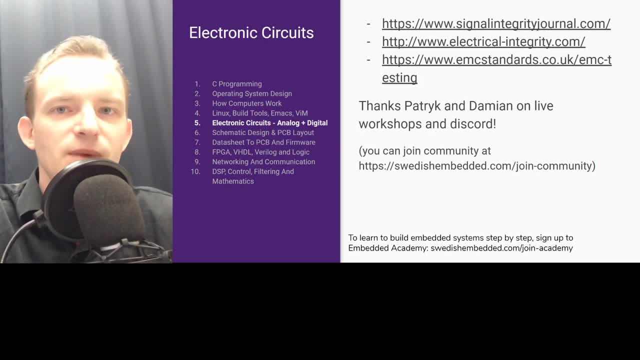 Except that when you move to the digital domain, when you start implementing everything in software, you're kind of implementing the same equations that govern the behaviors of passive components like capacitors, resistors. So you're doing it in the code domain. 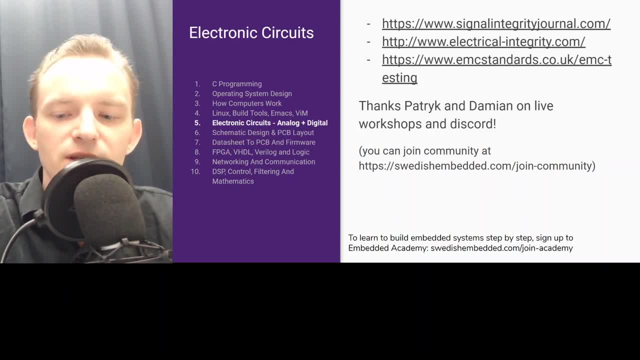 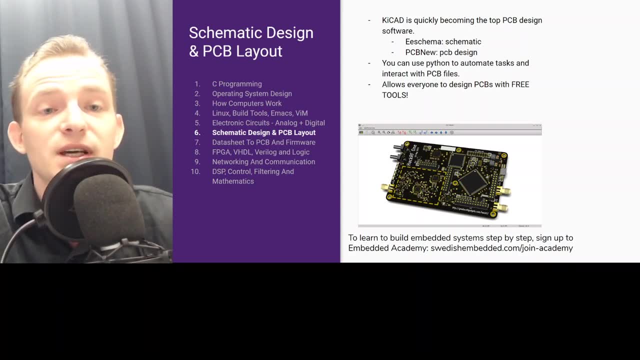 So it's really useful to kind of understand those areas. You want to get good at electronic circuits. You want to get good at schematic design. You have so many tools available to you right now. You have KiCad, which is getting better and better. 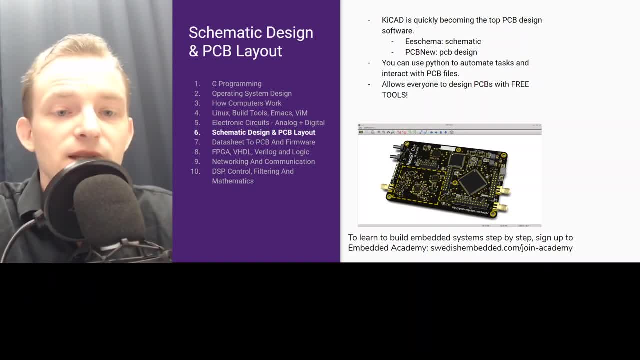 It's completely free And it's possible to create really complex PCBs using KiCad. This is, for example, HackerRef 1. And it's a fairly complex PCB And it's done completely in KiCad. So you have all those tools available to you. 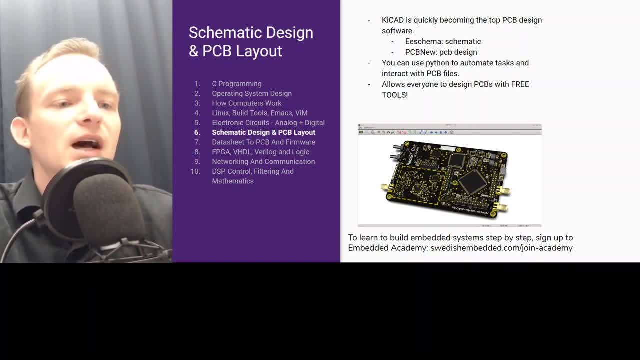 You don't even need to like. you can just download Linux. You can download all the build tools, text editors, You can download the PCB design software And you're ready to go Like. you can start creating products like this. 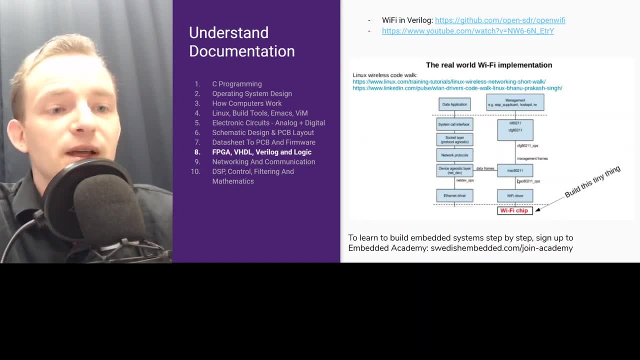 Eventually, you'll find that you want to kind of get better also at building digital circuits, Like when you want to implement something that needs to run really fast. A good thing to look into is FPGAs, And there's really cool projects that have been done using FPGAs. 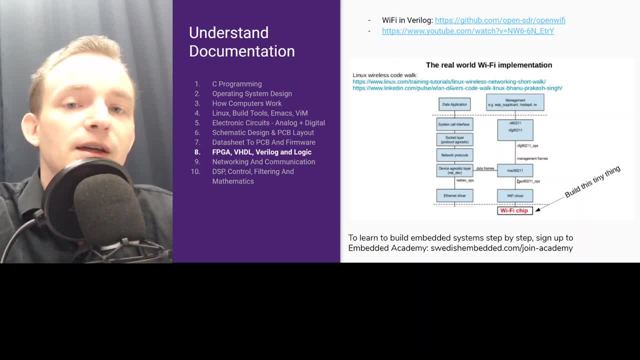 One of them is the Wi-Fi, the actual Wi-Fi implementation of a Wi-Fi chip done in hardware programming languages, And hardware really uses programming languages as well, Except that all of the algorithms you implement they're running really fast So you can implement like you're programming at a higher level. 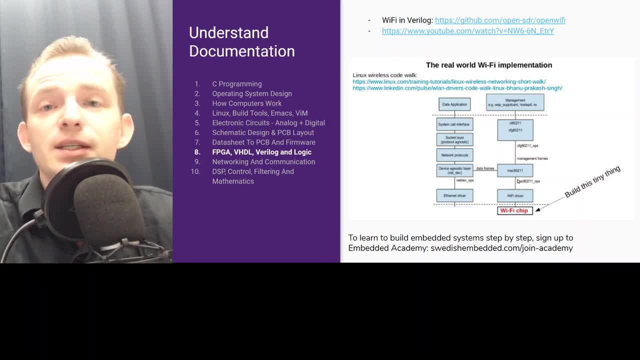 But what you program is getting translated into logical gates, So basically a digital circuit, And then you put it into a programmable logic chip where you can connect those gates using a programmable approach. So you can arrange those gates into your circuit. 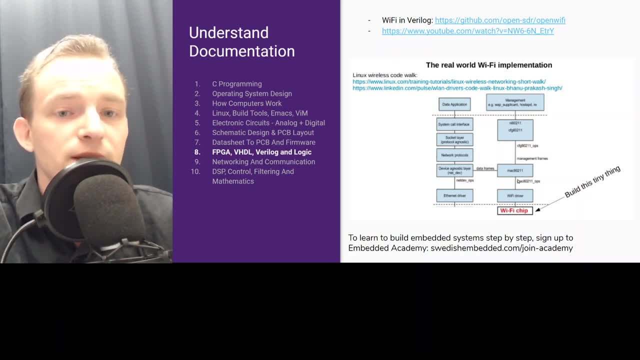 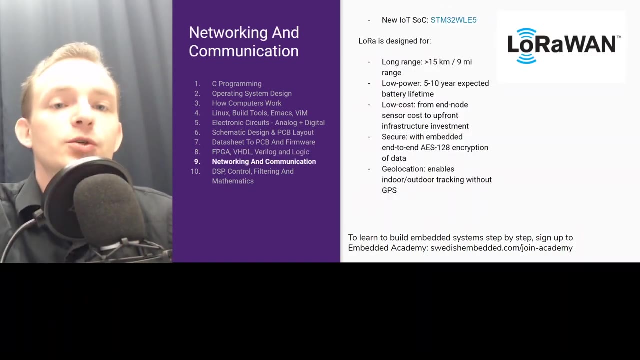 And once it's ready, it's going to run really fast Because you can literally execute things in parallel. Because it's just one circuit at every clock cycle, You can have many operations that take place And you want to learn networking. There's really cool solutions. 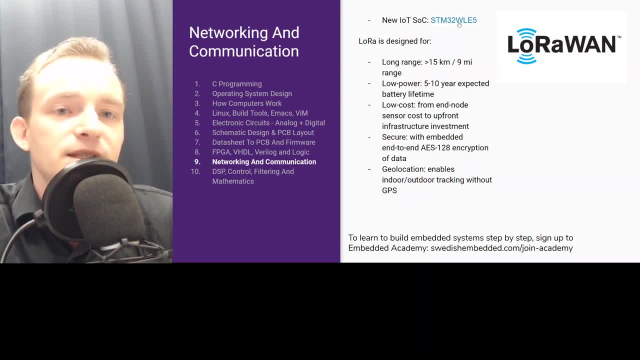 One cool chip that I found very recently is the STM32WLE5.. And it's actually a connectivity series of STM32s And I like STM32s a lot Because they're so powerful chips. They have all the profiles you need for most things. 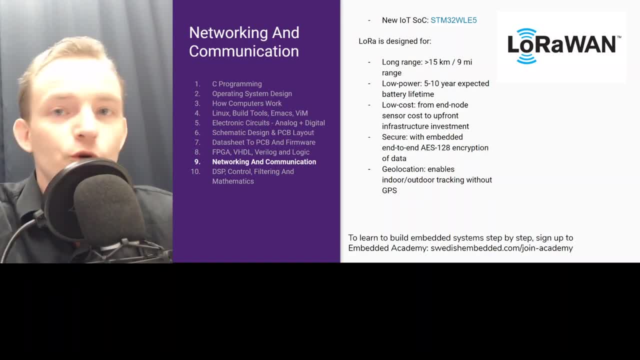 They are 32-bit controllers, So they're powerful. You don't need to jump through hoops trying to program like an Atmel controller, which is not a 32-bit controller Like 8-bit controllers. You kind of start when you go down into these lower-end controllers you start getting affected by the fact that the chip is not that powerful. 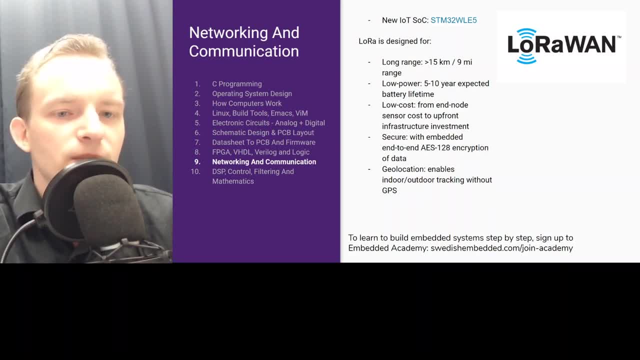 And that affects how you write code. So you kind of lock yourself out of using very useful abstractions in code Because your controller is so not powerful and not powerful enough that you have to optimize your code just for the sake of running it on the controller. 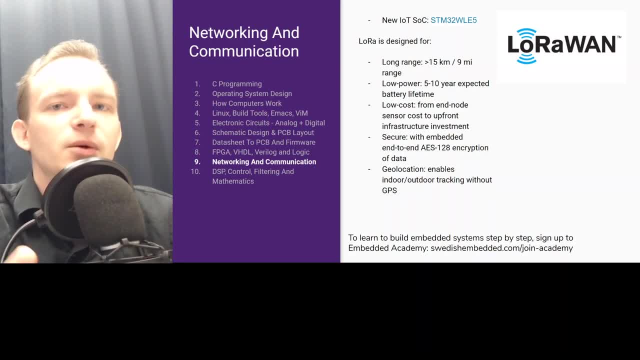 And I think that's wrong. I think it's better to have a chip that you can actually run real programs on, And STM32 is one of them. So this chip implements LoRaWAN. LoRaWAN is really cool. It's long-range. 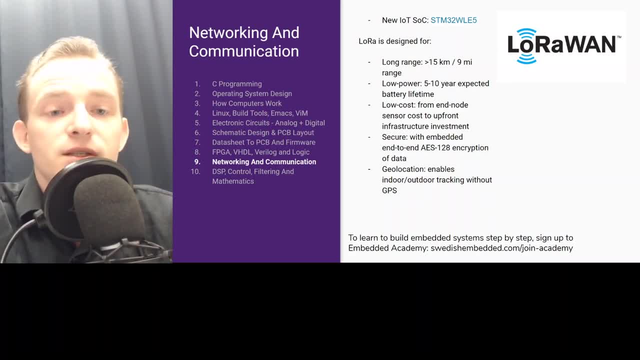 It's designed for long-range communication And it's designed for low power as well. It's really ideal for sensors that run on batteries and sensors that need to communicate over large distances. So definitely check it out and learn networking and learn communication, Because that's what everything is built upon. 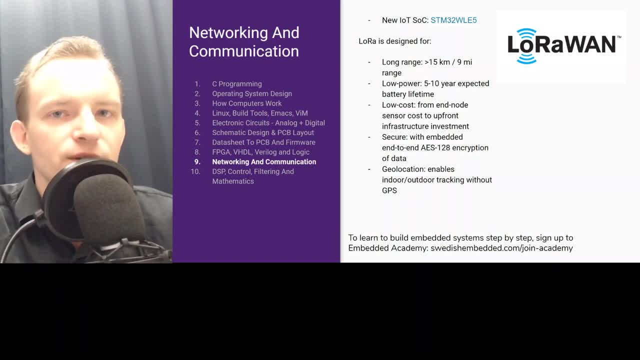 All the programs on the computer. when they communicate between each other they usually use sockets, Which is kind of similar to network communication, except it's happening between processes And all the messaging that happens between systems It's also done using communication. 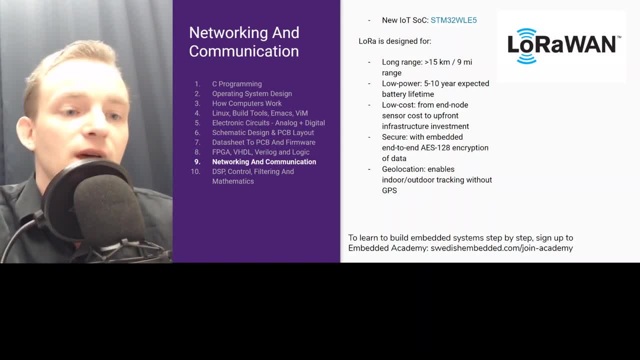 Either serial communication or IP communication And you want to get comfortable with that And really kind of get comfortable with using sockets for transmitting messages between devices. There's MQTT, for example, which is a standardized messaging protocol, So definitely check that out. 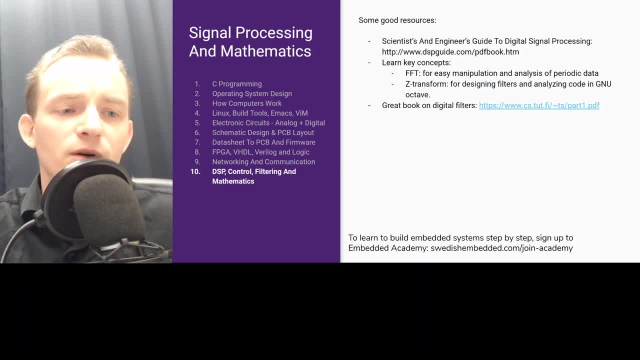 And finally, of course, the mathematics of digital signal processing, control theory, Filtering and anything else that kind of relates to the mathematical concepts. You'll find that it will help you. It will help you design your algorithms better, Because you don't want to be designing filters just by sort of trial and error. 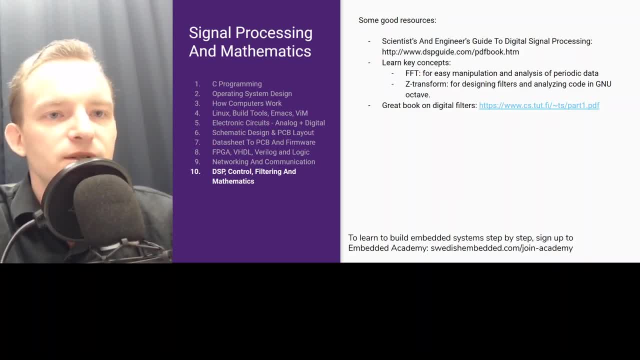 You're not going to be able to analyze them, You're not going to be able to really understand how the filter behaves at different frequencies, And so, digging down into DSP, I have a lot of resources. Here's a good book on digital filters, for example. 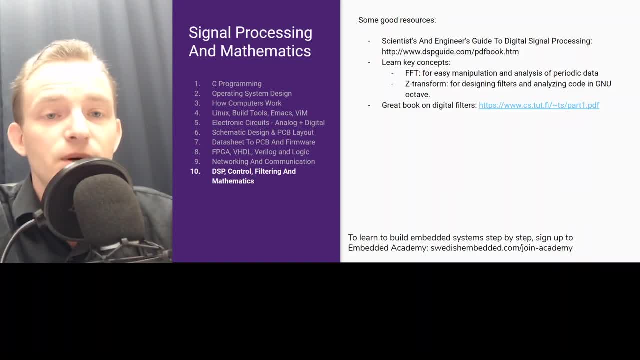 You can just go and read it online. There's also DSPguidecom which has a lot of material on the topics of DSP. digital signal processing- FFT, is really useful because it allows you to analyze a system, So you can feed a system with a signal of a composition of frequencies.